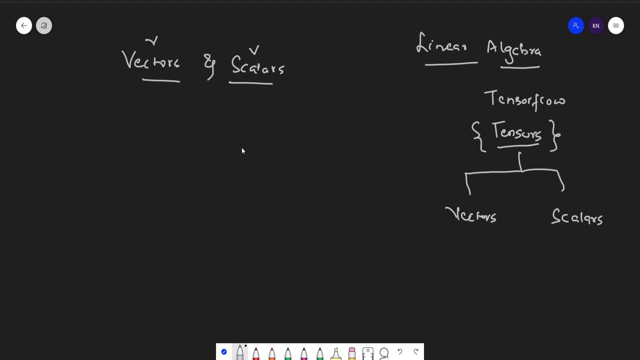 topic is really used in many fields, guys, let it be physics, chemistry, maths. you know, in every most of the major subjects this quantity is really used. Now, vectors are scalars. before going ahead with this, guys, let me just first of all discuss about scalars, Scalars and 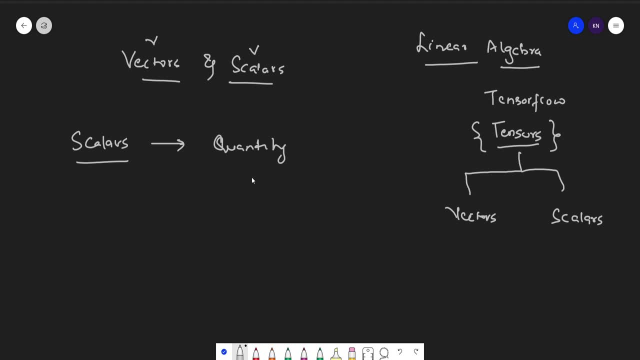 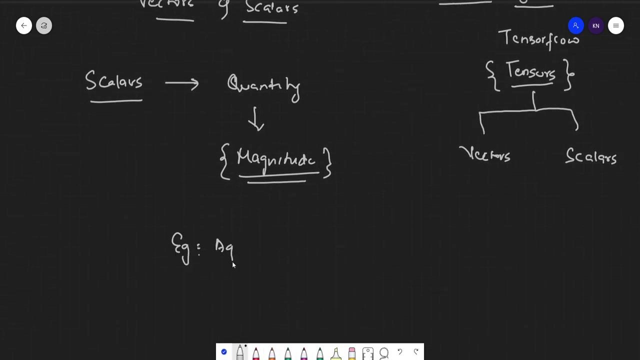 it is a quantity. it is a quantity That has some magnitude. Now, what exactly is this magnitude, guys? let me take an example. Suppose I say age- age of a person. or let me take a much more simpler thing: Suppose I say speed of a car In speed. 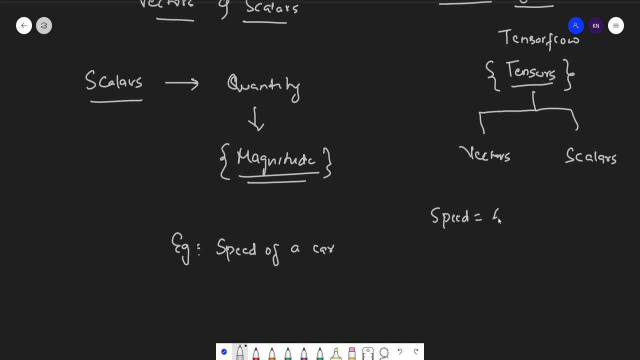 of a car, I, we basically represent it as 45 kilometers per hour. So this is basically the unit and this is basically called as the magnitude. the magnitude is represented by this particular unit. okay, now, scalar is a kind of quantity that only has a very important property, which is called as magnitude. okay, but if I go, 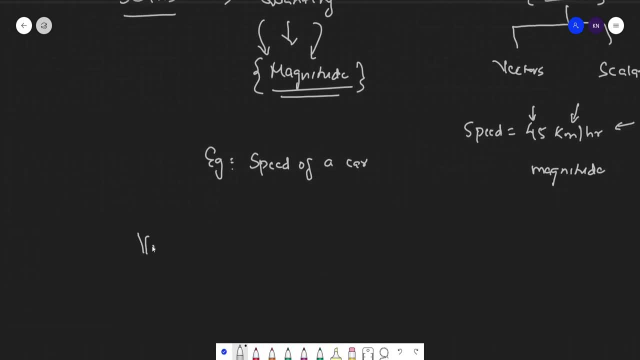 and understand about vectors, you know so in vectors it has two important properties. so it is a kind of quantity which has two important properties. one is magnitude and the second one is basically direction. now if I really want to give a good example for this, I may say that the car is traveling east at 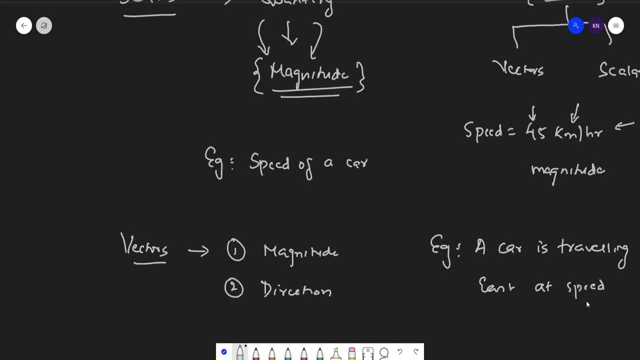 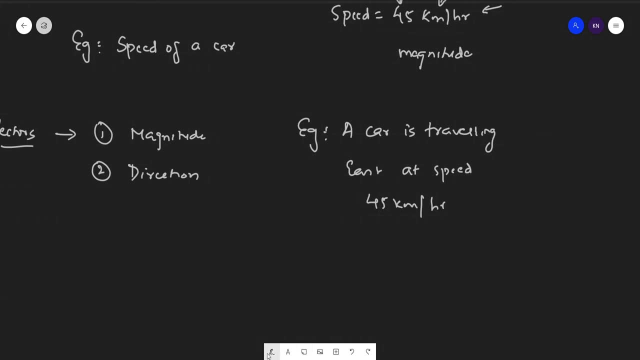 the speed of 45 kilometers per hour. now when I write this kind of example, guys, here two important information is basically getting convert. one, they have actually told a direction. the other one that they have actually told is speed. so over here the magnitude that has been shown you know. so let me just write it in a better way. 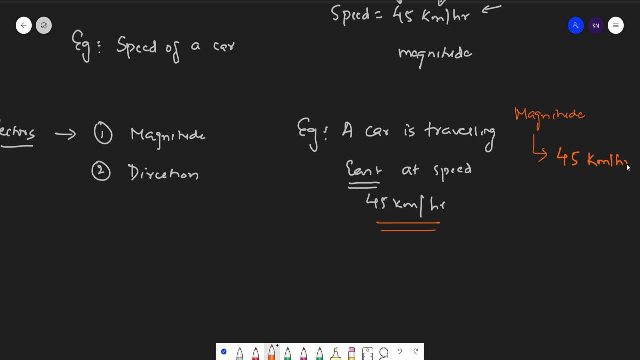 magnitude over here is nothing but 45 kilometers per hour, and here the direction is also shown as the magnitude of the car. so this is the magnitude of the car. so this is the magnitude of the car. so if I say that this is the esquire, I get shown. 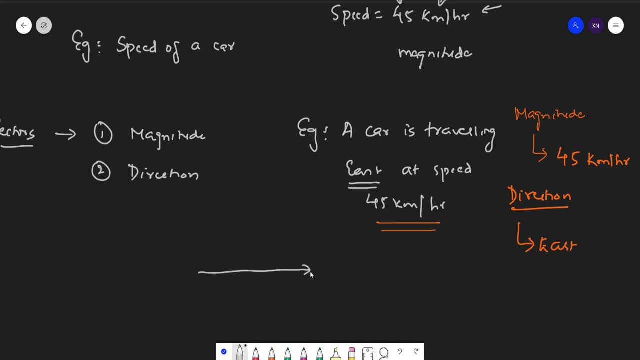 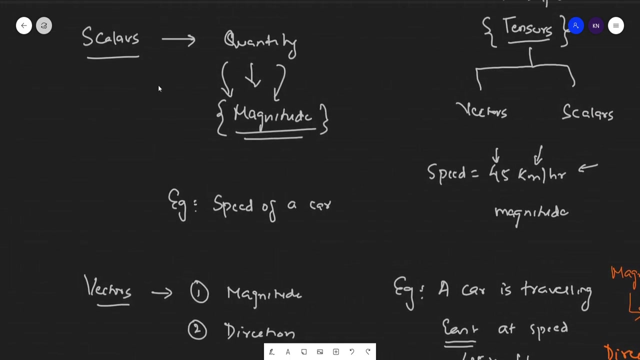 okay, the direction is basically east. okay, so in that, if I really want to draw it diagram, butter meant濃 suppose. if I say this is east, the car is basically traveling at the speed of 45 kilometers per hour. right? so this is the basic difference between scalar and vector. if anybody asked you about what is a scalar, 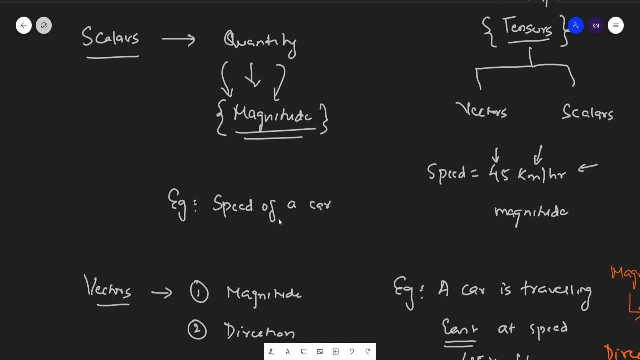 you can definitely say that it is the quantity that actually has some kind of magnitude. example: a speed of a car. you can definitely say that it is a quantity that actually has some kind of magnitude. example is speed of a car. I may also say that you know the distance, the distance between two people, that they are. 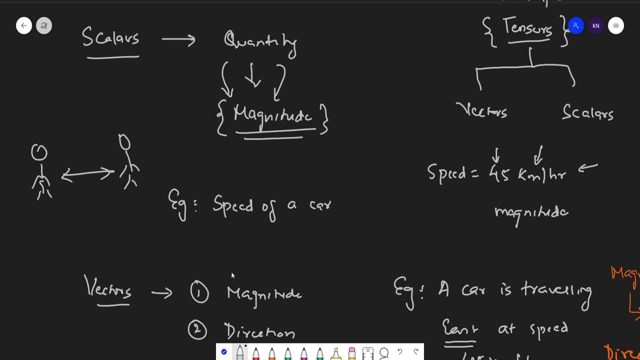 standing. okay, what is the distance between them? and many more examples like how many liters are basically present inside a jar, or what is the bottle size? probably you may be saying that it is two liters, it is three liters, all these things right, but whenever we talk about vectors, 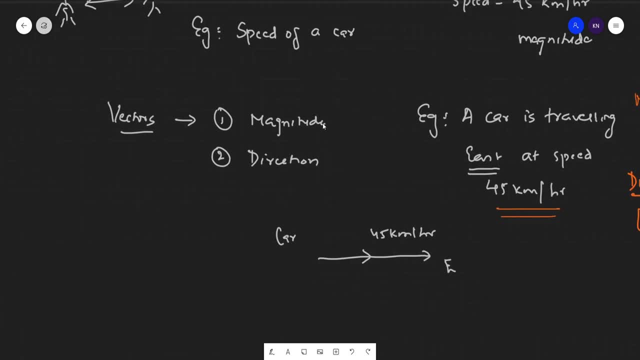 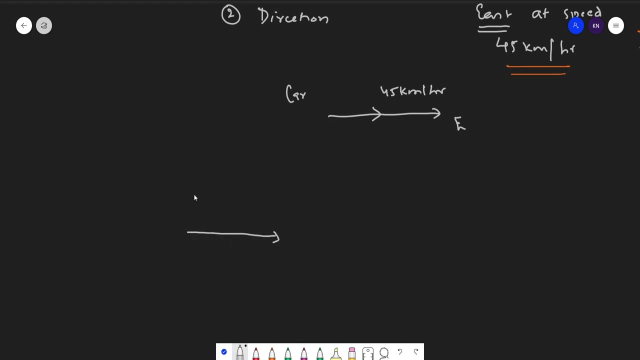 we definitely have to discuss about both thing, that is, magnitude and direction. So this was one example. okay, the car traveling at a speed of 45 kilometers per hour. not only this, guys. now let's see how mathematically or graphically it is basically represented. Suppose if I have and 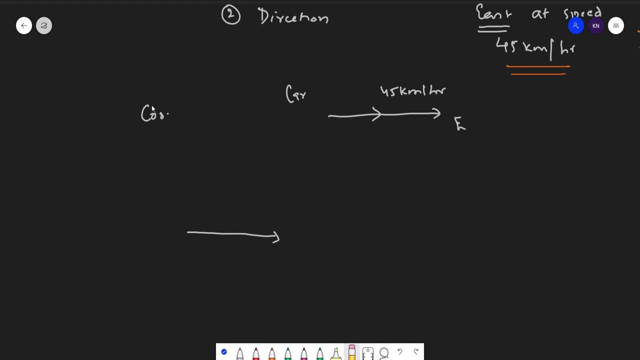 usually for vectors. if we really want to represent it diagrammatically, we really need to use something called as coordinate spaces. okay, Now, what is the coordinate space? Now, what is the coordinate space? Now, what is the coordinate space, this coordinate basis, suppose i hope everybody have known about this. x and y axis, right? sorry, 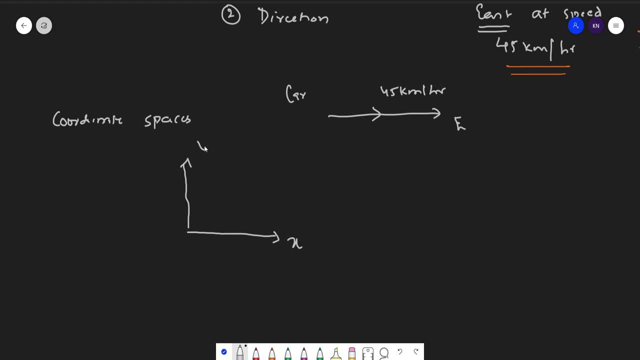 for this. so suppose this is my x and y axis. okay, and this side, obviously, when, if i go this side, this will be negative x, this will be negative y. okay, so i'll just write over here as x bar and this will basically be my y bar. okay, let us represent: this is my x? uh axis. this is my y axis. 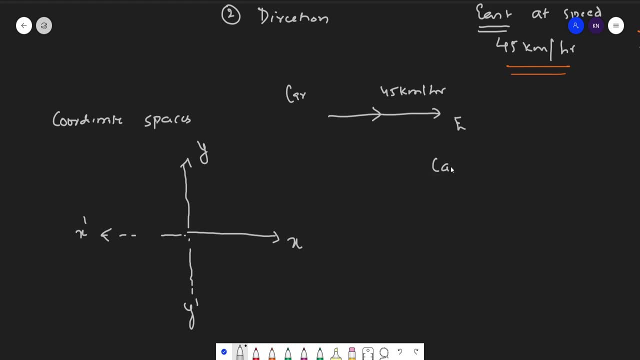 now suppose, if i want to say that the car is traveling at the x direction, okay, so we basically mentioned this kind of this kind of arrow. you know, it can also be represented as x bar. this is how a vector can be represented. okay, so, since it is going towards the x direction, 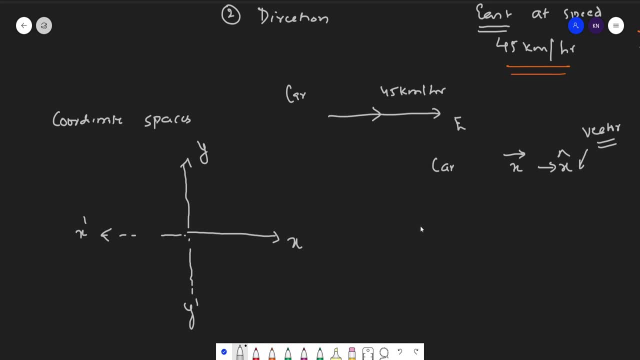 uh, probably at a speed of 30, 40 kilometers per hour, right? first of all, how do we represent this particular x axis, you know? so we represent it with some unit vectors. okay, some some values over here, right. so over here the unit. uh, we basically have two main important properties. whenever i say 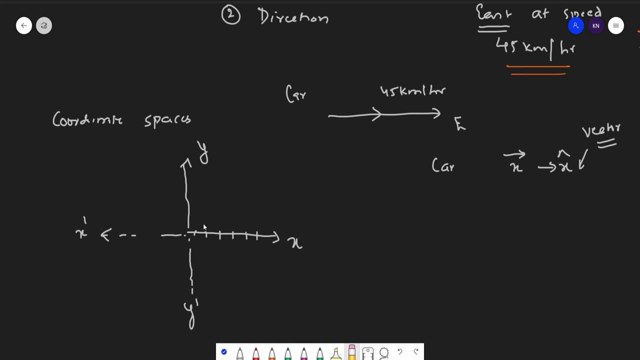 you know whenever, whenever we say, uh, that the car is basically traveling in this direction. okay, the car is basically traveling in this direction. so here we know what may be the magnitude. suppose we say that the car is traveling at four kilometers per hour. when it is traveling at 4 kilometers per hour. 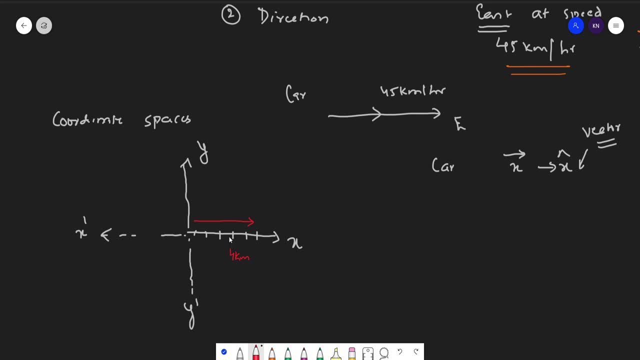 hour, right? so we have definitely represented in the form of unit magnitude, right? so? unit magnitude, like this one unit is one kilometer, two kilometer, three kilometers, four kilometers. so from here to here, this is basically my four kilometers, right? so this, this entire thing, is my four kilometers. so if i go and represent this specific value, i can definitely represent. 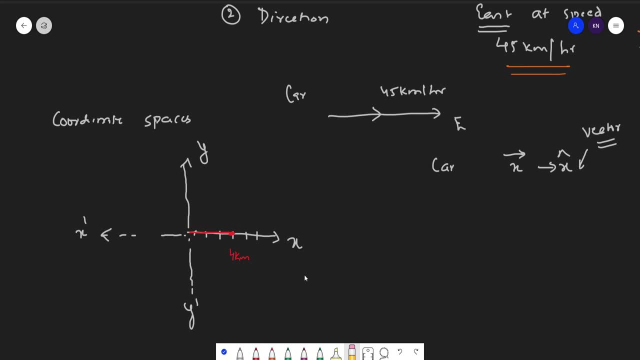 this: suppose the car is moving at this particular direction, i can definitely represent it as four x power. okay, so this is how i will represent this vector quantity. okay now, similarly, what i may do is that i may also have my y-axis one, two, three, four right and five, then six, suppose i say. 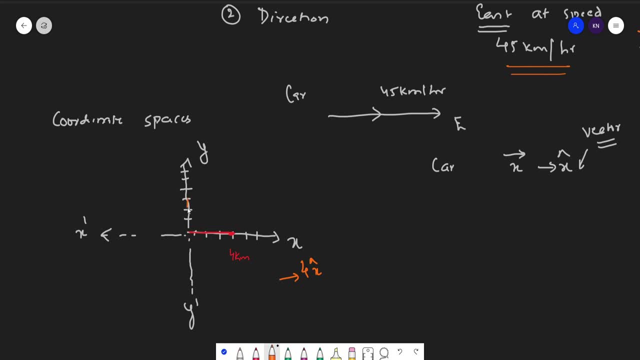 that the car was moving three kilometers on the y-axis. so this is my one, two, three, okay, three kilometers per hour. so I can represent the speed you know in the y-axis. so probably i want to represent, if i'm representing a vector quantity, i will represent in the form of y bar, okay. so suppose if i say this as three, 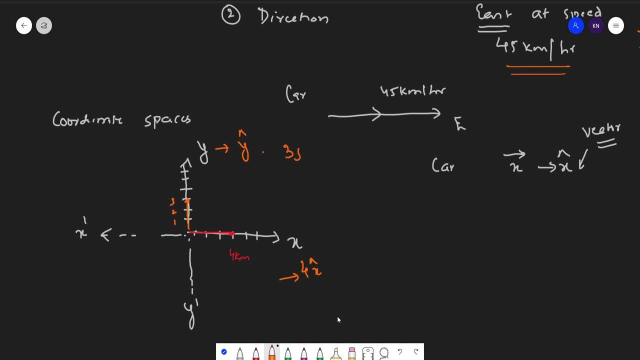 then i can represent this entire value as three: three x bar, okay. three x bar, sorry. three y bar, okay. so here i have four x bar and three y bar. so that basically means, if i really want to find out how this particular movement was happening, can i not make a simple point: where these two points are actually meeting in this two-dimensional space? it is meeting somewhere here, right? 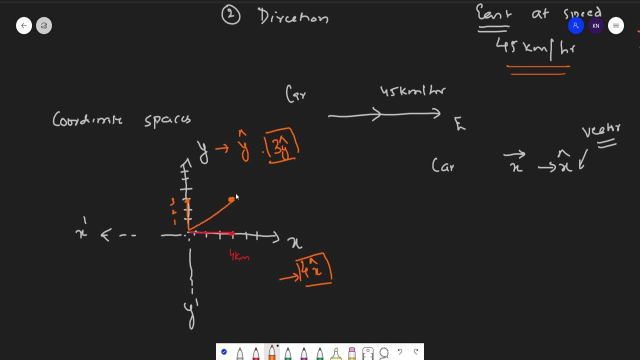 and this entire distance can definitely be calculated. if i just use a pythagoras theorem, i may make this: aso this man be a and this may be my b, so this is obviously my pythagoras theorem. i can basically use o. a square is equal to. I can basically write OB square plus AB square. this is what my Pythagoras theorem. 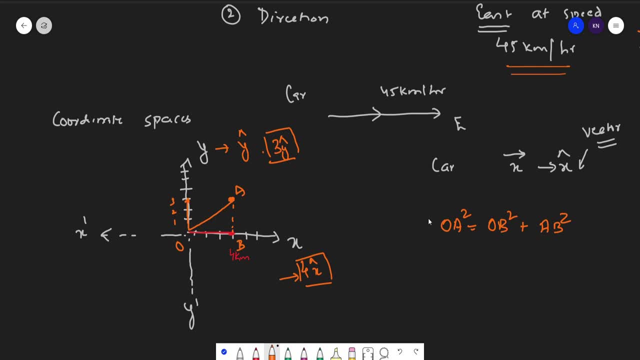 actually says right and based on this I can definitely calculate my OA square. but over here you can understand. one very important thing is that if I really want to represent this particular point, it can be represented in the form of 4 comma 3, or this can also be represented as 4x bar. 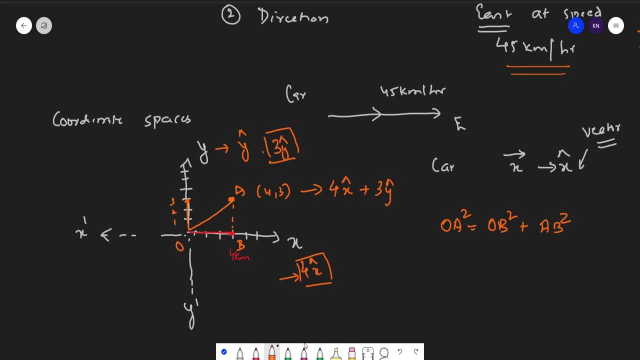 plus 3y bar and suppose, if I really want to represent this in the form of linear algebra, so probably in the form of array or matrix, I can basically represent it as 4 and 3, right? something like this. I hope everybody is understanding, right? this is how vector. 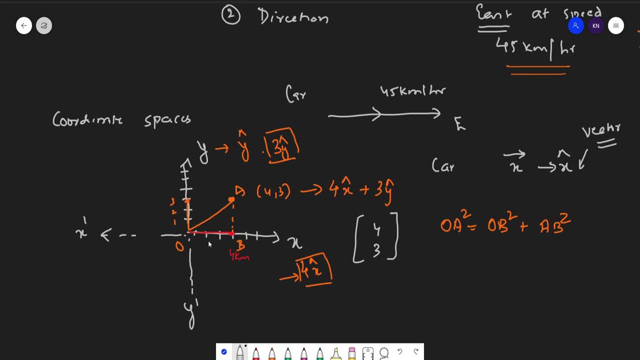 quantities are basically specified. you know, if I, if I show over here, suppose this particular vector is basically moving 4 kilometer, 2, what's the x-axis? 3 kilometers towards the y-axis. so this can basically be represented by this particular point, which we can actually represent with this 4x bar plus 3y bar. and then, if I really 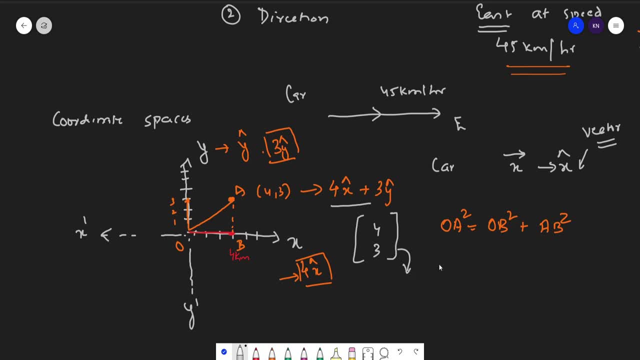 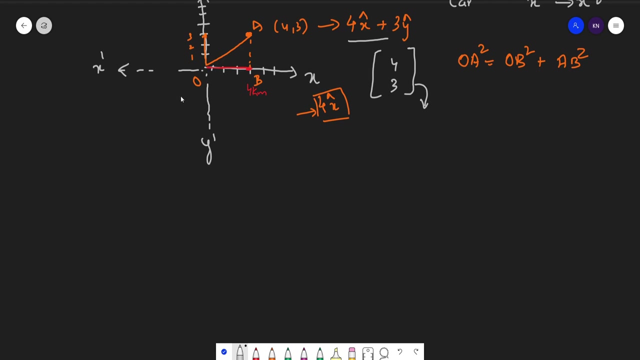 want to represent in the form of matrix. it will be 4 comma, 3 matrix or array, okay, so this is how entirely we represent the vectors. this is very, very much important. now, always understand one more thing, guys, one very important property about this: this, this vectors. you know, suppose I have there is a two people over here. okay, two people over here. 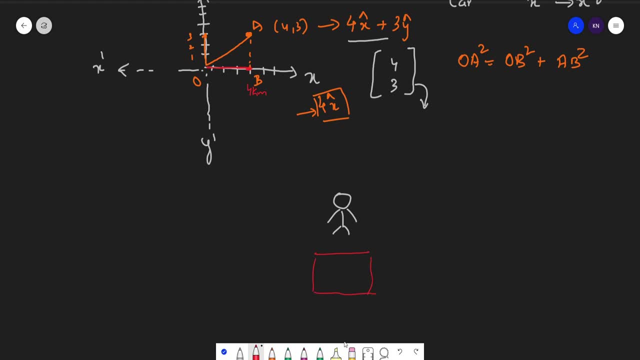 and they really want to move this particular object. right, move this particular object. suppose there are two people's over here. if they really want to move this to particular this object. okay, from here, basically to here. okay, because this will be very much important, because it will make 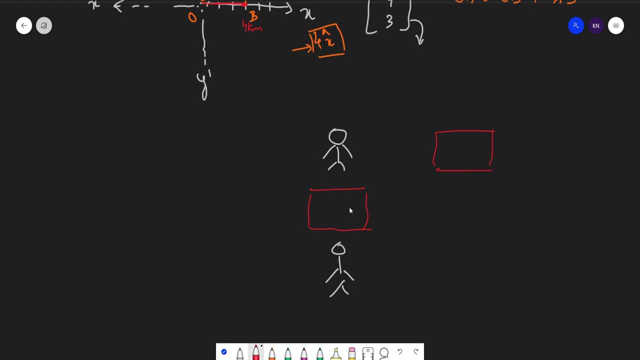 sense, guys, trust me. okay, now, if this particular objects needs to be moved from here to here, then usually we will be following this direction. right, and in order to follow this particular direction, just imagine that we have taken this direction, we have taken this direction and then we have taken this direction. 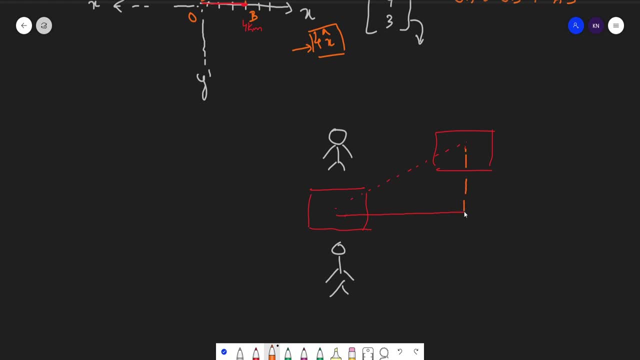 okay, we have taken this direction. okay, now just understand the movement of people. you know so. first this person will be moving in this direction, and then this person will be actually moving in this particular direction. then he will be moving in this direction. similarly, this person will also be moving in this direction, he will be moving in this direction and he will also be moving. 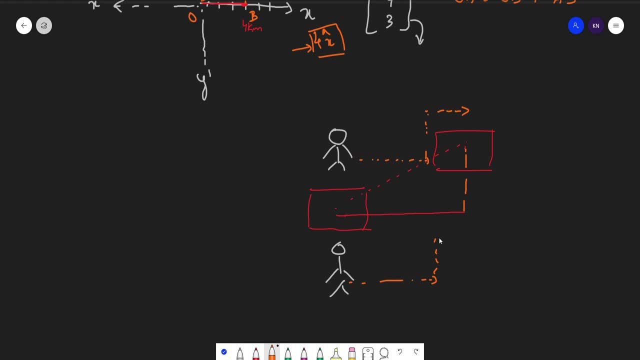 in this direction. okay, or I can just increase this over here like this: and he will be moving in this direction and finally, when they come to this particular point, you know, here you will be able to see that they will be placing this particular object. okay, one very important thing about this specific movement: 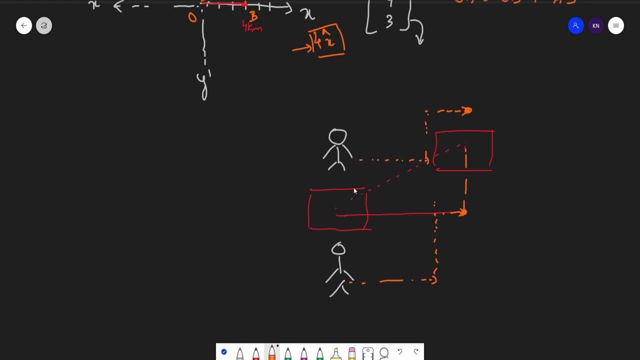 that you will be seeing. you know, when these two people are trying to pick up this particular object and place it in this particular position, both, this particular person, will be having the same type of movement. okay, they will be having the same type of movement. okay, same type of movement. so here you can see that this particular movement of vectors is also same. 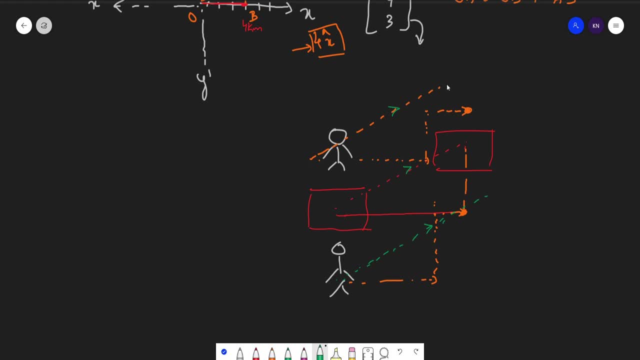 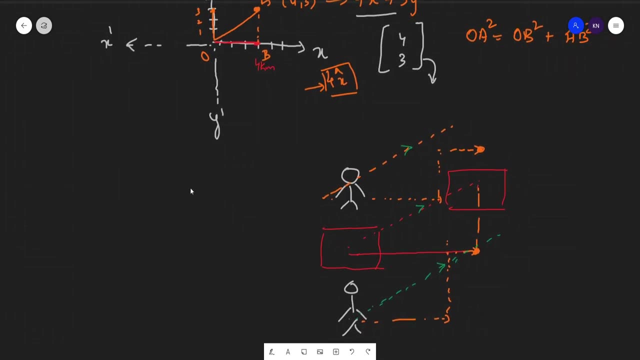 movement of the all these three vectors, how the object is also moving, how the people are also moving- this will be almost same. so one very important thing that i really want to convey from this particular example is that if the movement of a specific vector is in their 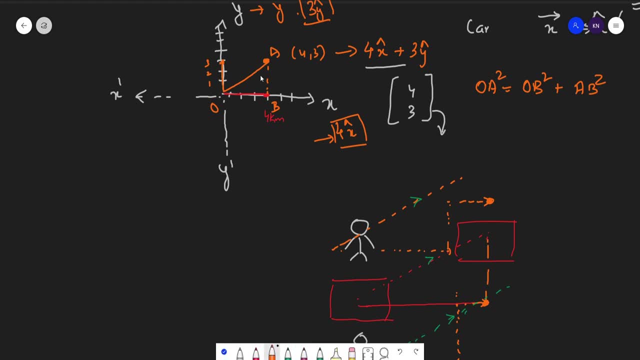 direction. if i try to create some other vector which will also be over here, which will also be over here, which can also be over here, which can also be over here, the type of movement, the type of vectors will be almost same. that basically means i can also represent this particular. 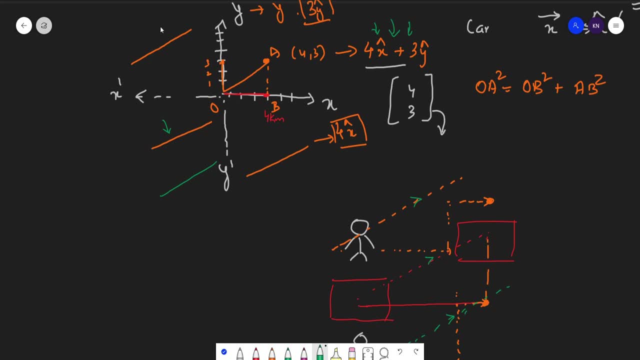 vector with the same equation. okay, i can also represent this particular vector with the same value, you know. so we can definitely represent it with the same value. the only thing that is changing is basically your origin, basically your origin, right? so this vector is almost equal to this. this vector is almost equal. so these all are the similar vectors, because 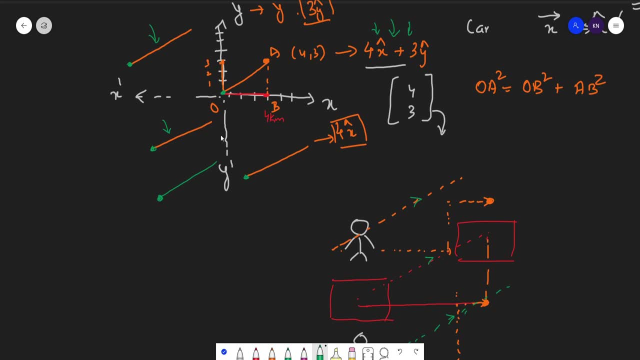 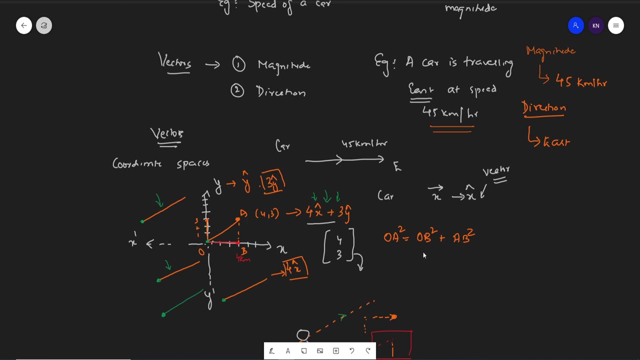 you. they are in the same direction. they are in the same magnitude, right? The magnitude is almost same, right? I hope everybody is able to understand this, okay, So I hope you like this introduction session about vectors and scalars, And trust me, guys, I hope this will be very much important. 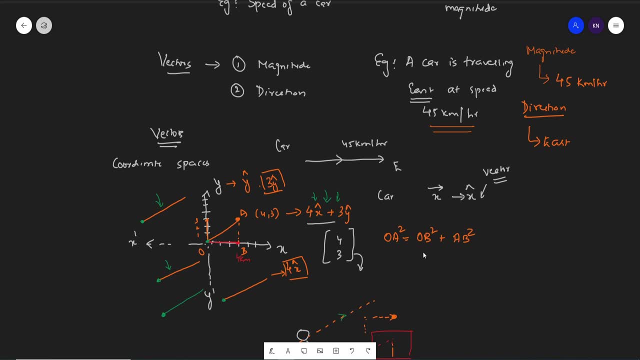 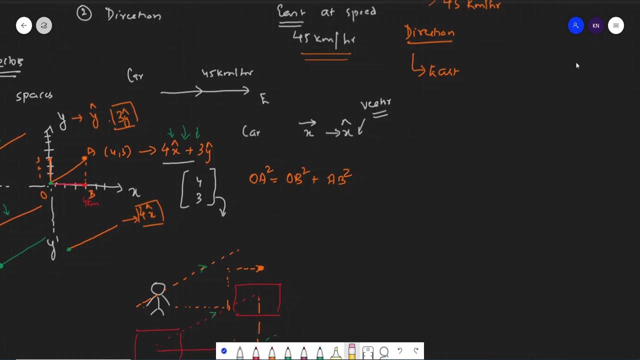 in data science. because in data science, in machine learning, suppose, if you're solving any machine learning problem statements, right, What is the most important thing in machine learning problem statement? There also you have features right. There also you have features right Like this: F1, F2, F3, F4, F5, you know, and probably one output feature. 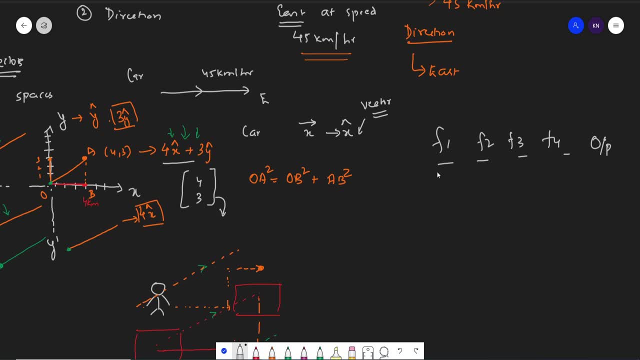 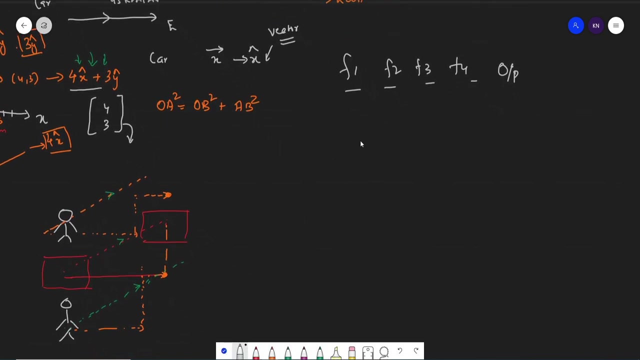 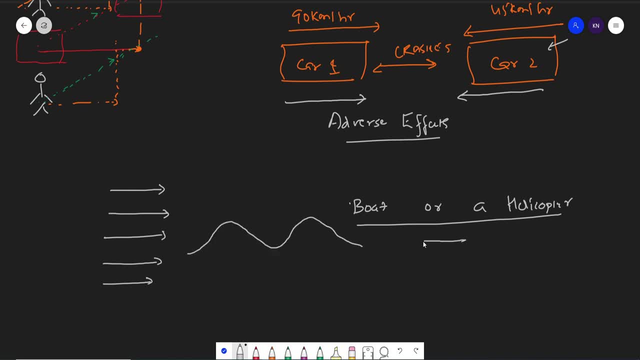 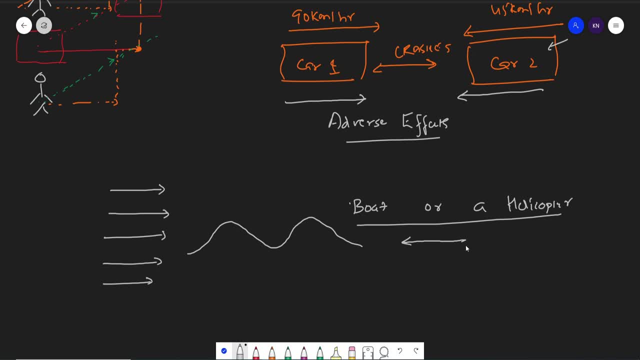 boat will go up. suppose if you're, if you're driving your boat, if you're riding your boat from this direction, then you what may happen? it may go up, then again it may come down. right now, suppose what if you have a scenario- and this is how, how this adverse effect is basically created. 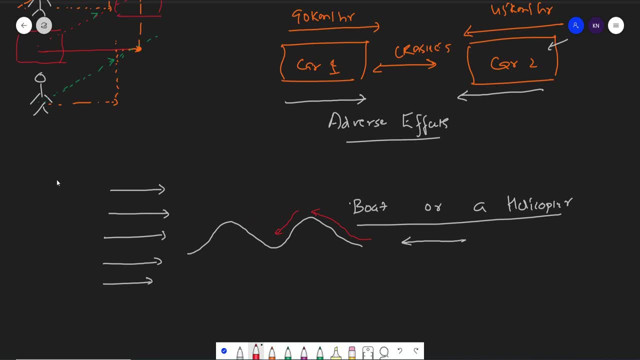 because of this particular direction. they're trying to come up with some outcomes based on this particular vectors, right? not only this. suppose, uh, the wind is actually flowing over here and there is another wind that is flowing in this particular direction. now, in this particular scenario, if you see some games right over there, the cyclone will get created. i'll not say cyclone. 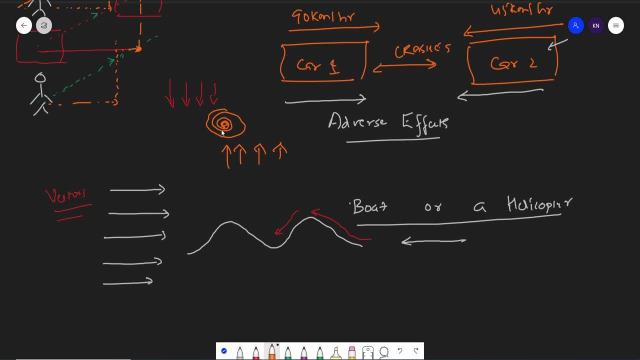 but instead a whirlpool inside the ocean may get created because this, this, this winds will be flowing in this direction. then, right when, when two winds intermixes, right. so these are another outcomes that can be caused by this kind of vectors. now, what is the vector over here? 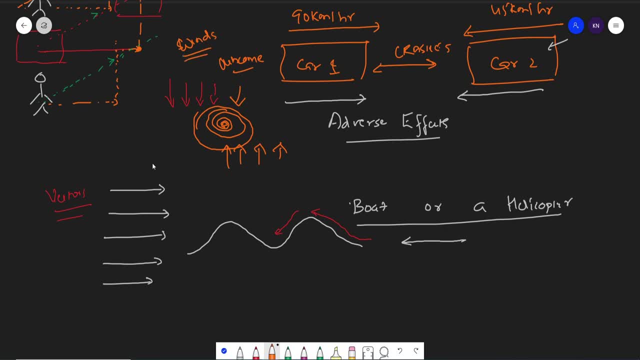 wind which is flowing at some specific speed and in and in in programming also, they may write a condition if the wind is probably flowing at 45 kilometers per hour or not. so whatever units we use, and probably this wind is basically traveling for 100 kilometers per hour. now what will happen?